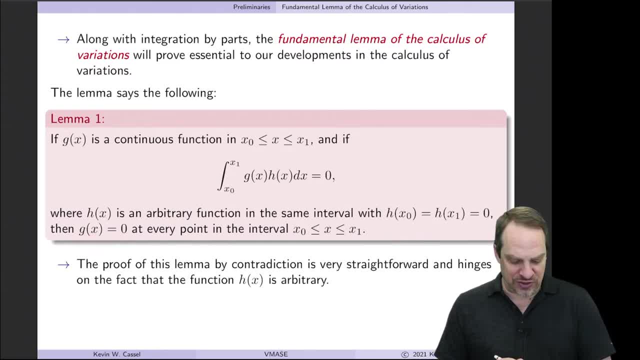 be satisfied that integral is if g of x is equal to 0 over the entire interval from x0 to x1.. So again, we're going to prove this by contradiction, which means we're going to prove something that's true by proving what can't be true. So let's suppose that 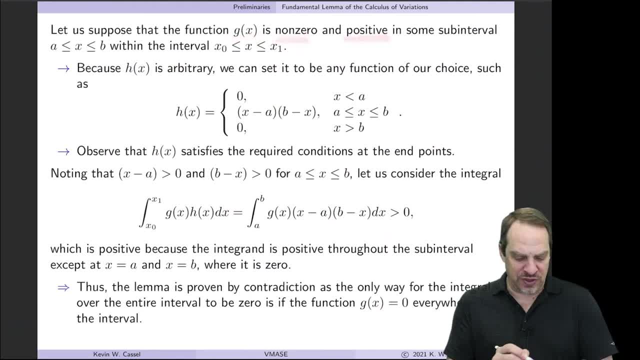 the function g of x is both non-zero and positive in some subinterval from a to b, within the interval x0 to x1.. And what we're going to show is that by making that assumption, this lemma cannot be satisfied. So therefore the opposite has to be true. In other words, we'll show that g of x has 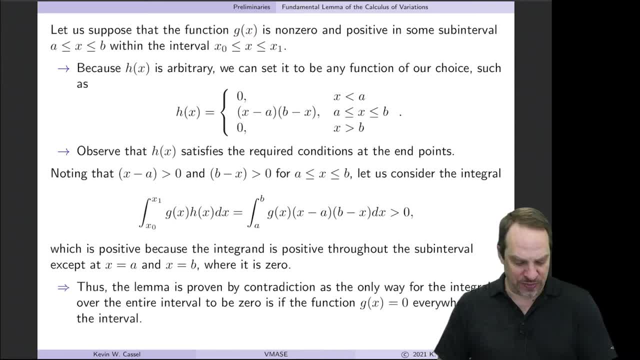 to be equal to 0 across the entire interval. The whole key is the fact that h of x is an arbitrary function. So we don't know what h of x is. It can be any function. It has to be continuous, but it can be any function between x0 and x1.. If it's arbitrary, I can. 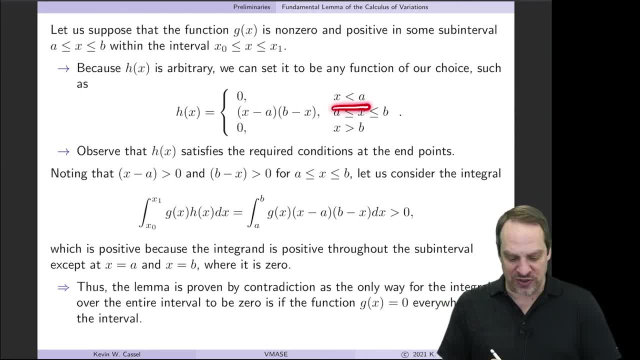 choose it to be whatever I want. So let's choose it such that, for x less than a, h is 0.. For x greater than a, h is 0.. For x greater than b, it's also equal to 0.. And it's only in this interval from a to. 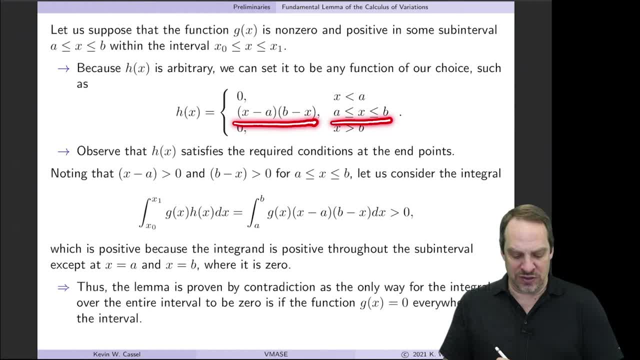 b that it has non-zero values, x minus a times b minus x. So essentially it looks something like this: Here's a and b, and it has a parabolic form: 0 before and 0 after. Now you'll notice. 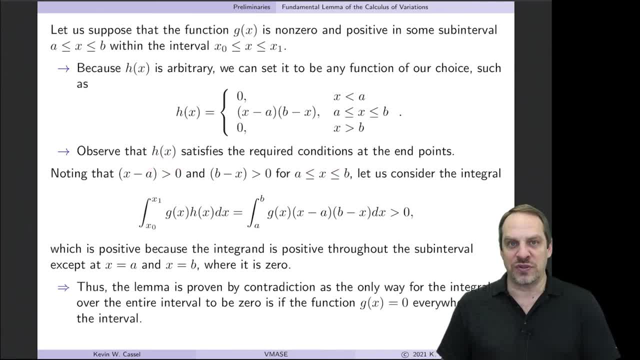 h of x satisfies the required conditions at the endpoints. So we haven't violated that. Now x minus a is always going to be greater than 0. b minus x will also always be greater than 0 in this interval, x going from a to b. So 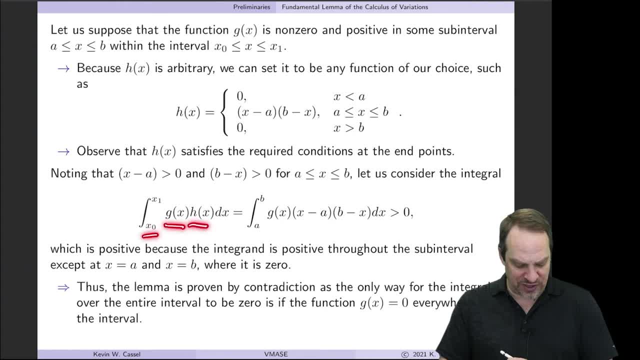 let's take a look at this integral: integral of g of x times h of x, from x0 to x1.. Well, if h is 0 for x less than a and 0 for x greater than b, then the only contributor to the integral 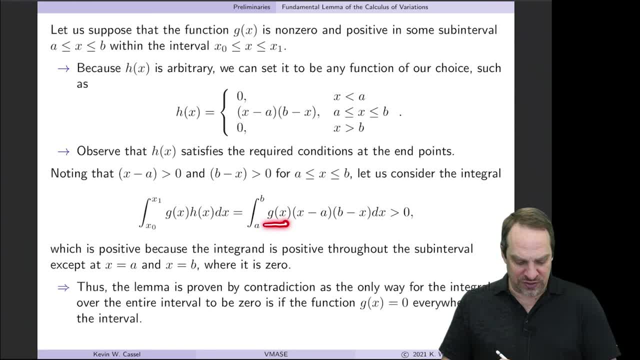 is going to be from a to b And that's our g of x, which we said is non-zero and positive. So if h is 0 for x times x minus a times b minus x, that will be greater than 0. We said: